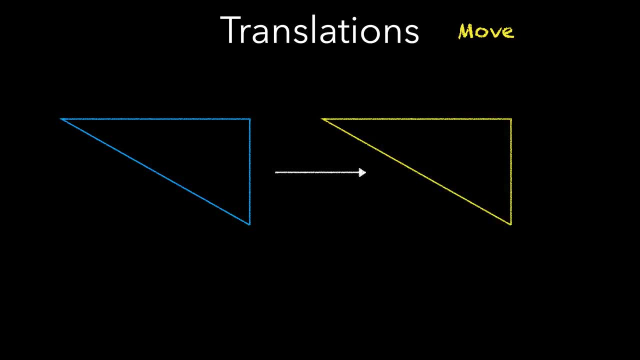 It stays the exact same size. the angles are exactly the same. it just moves. A reflection is going to mirror the shape, So the shape stays exactly the same, it just mirrors itself. So you draw a line of symmetry and then each shape is equal distance from that line of symmetry. 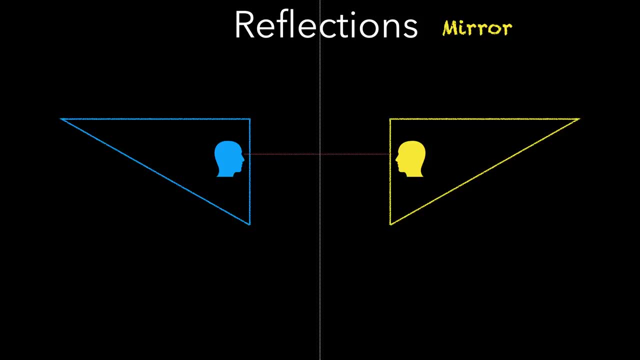 and it's looking right back at itself. That's what a reflection is. A rotation just rotates, So all the angles in the shape will rotate a certain amount of degrees like that. So I'm going to go over here. we're going to have some translation reflection or rotation pop up. 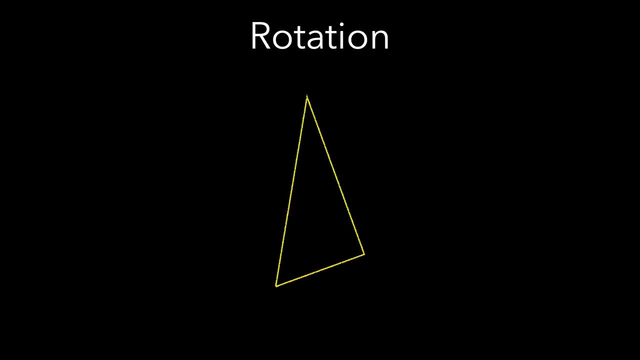 and the shape will do what it says. So here it's a rotation. so the shape is going to rotate, Now it's going to transform, which means it's going to move, And now it's going to reflect, which means it will mirror. 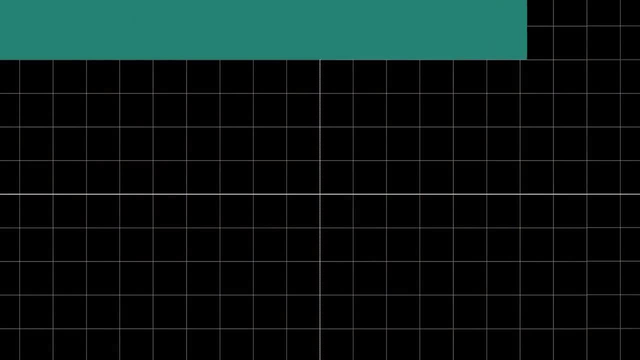 Alright, let's look at what it looks like on a grid, And the instructions will be in this green part at the top. And so let's start with the shape and let's give it some instructions. Transform the shape three units to the right. 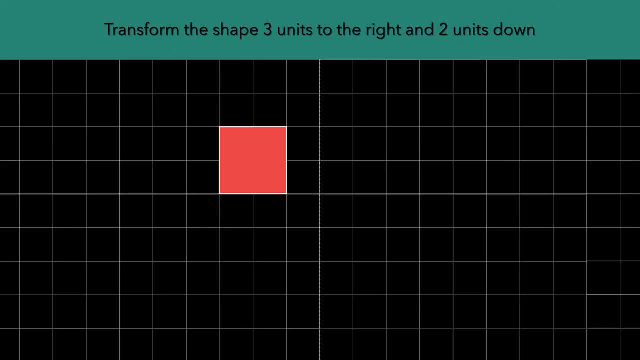 And two units down. So we're going to move it three units to the right And two units down, And that is So. here's our triangle, And let's see what the instructions say. Transform the shape: five units to the left and four units up. 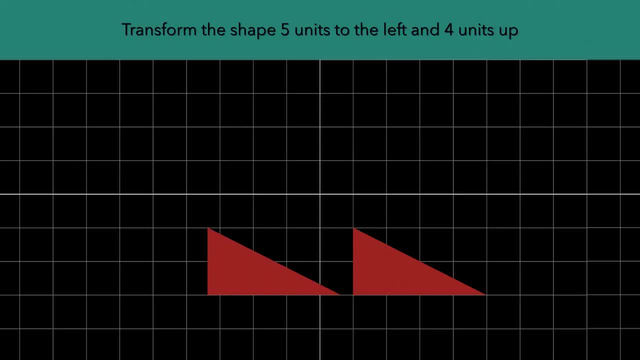 So let's move it five units to the left. There's five units to the left and now four units up, And that is the new transformed shape. Again, notice that the shape is exactly the same as the previous shape. It just has moved five units to the left and four units up. 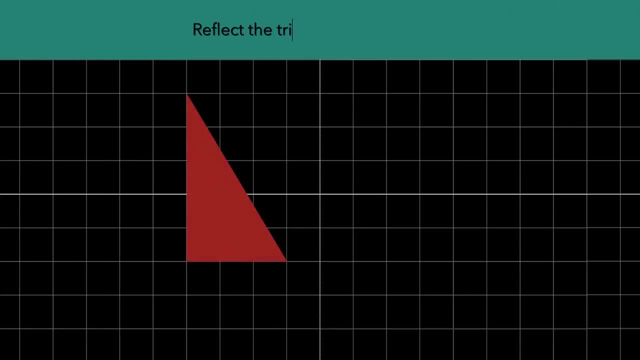 Let's try another triangle, And the instructions say to reflect the triangle over the y-axis. So we see our y-axis right in the middle there And we're just going to reflect it right over that. That y-axis will be our line of symmetry. 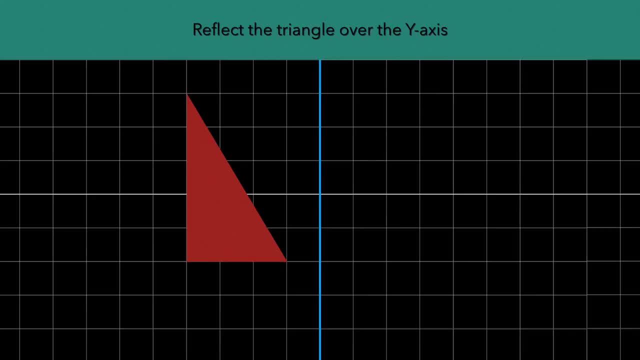 So let's reflect it equally from that y-axis And see how Notice each part of the triangle is the same amount of distance from the line of symmetry. That is the key in reflections: Each shape has to be the exact same distance from the line of symmetry. looking at itself. 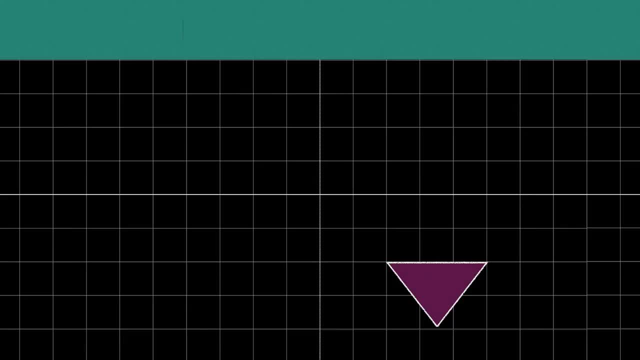 Let's try another one. Reflect the triangle four units to the left. So that's a little confusing, but that means we're just going to find our point furthest to the left, Our angle furthest to the left, And count four units to the left. 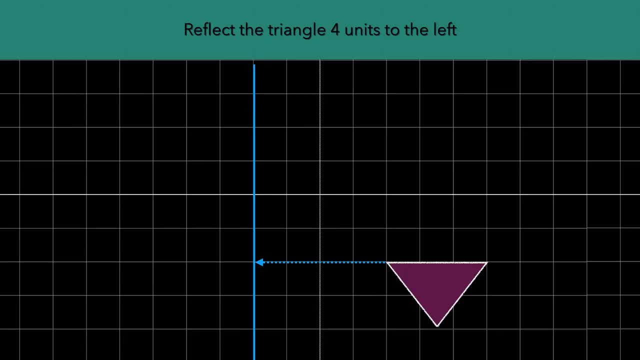 And that is going to be our line of symmetry. right there, That's our mirror And that means we're going to do the exact same Uh Uh For the. The reflected shape is going to be the same amount of distance from that line of symmetry. 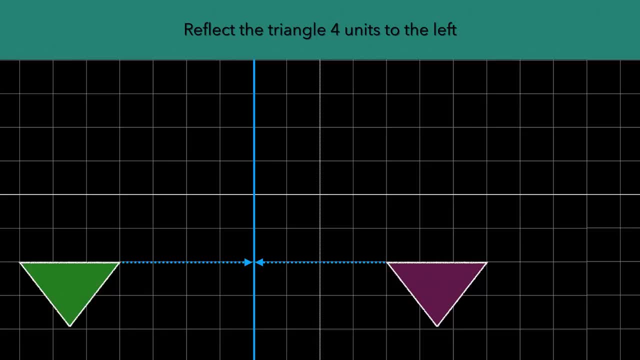 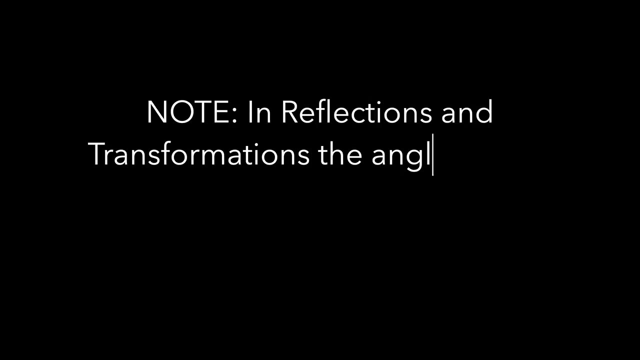 So it's four units away from that line of symmetry. And that is our reflected shape. Notice it's exactly the same And it's the exact same distance from the line of symmetry. Uh, And here's something to take note of: In reflections and transformations, the angles of the shape do not change. 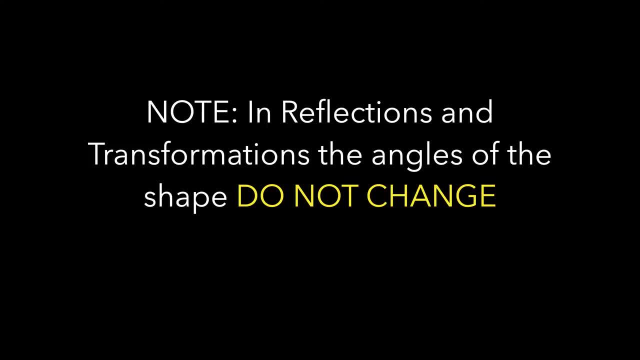 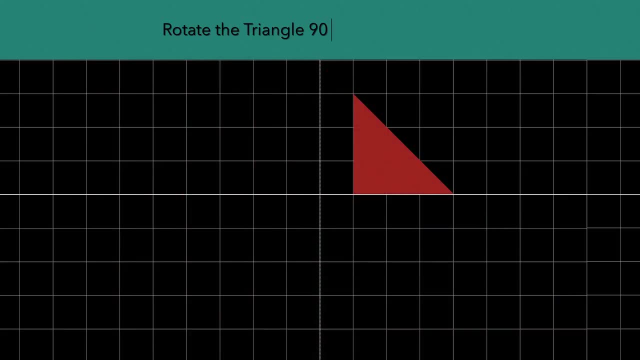 So write that down, screenshot, whatever you need to. In reflections and transformations, the angles of the shape do not change. Let's go over another shape with more instructions. So this says: rotate the triangle 90 degrees clockwise. So what does that mean? 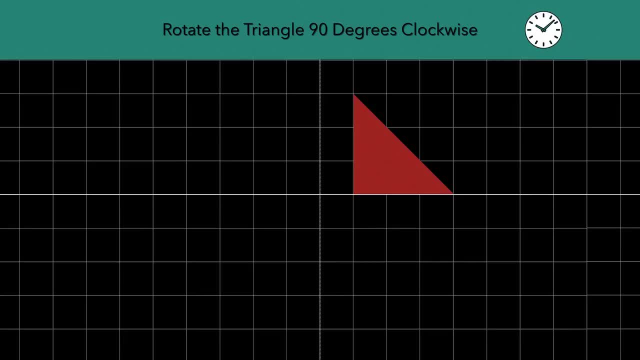 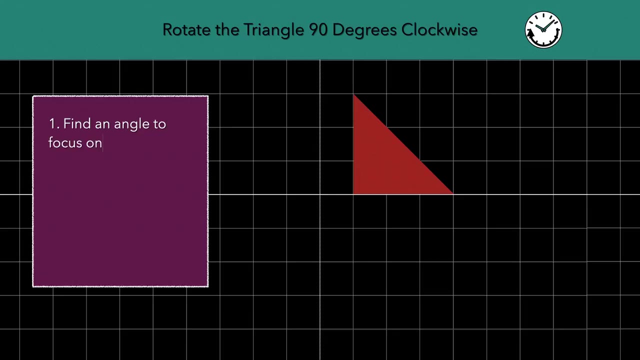 Clockwise, it means it's going to rotate, the same way a hand on a clock rotates. So that's going to go that way. Uh, So here's some instructions when doing rotations. Uh, The first step is you find an angle to focus on.